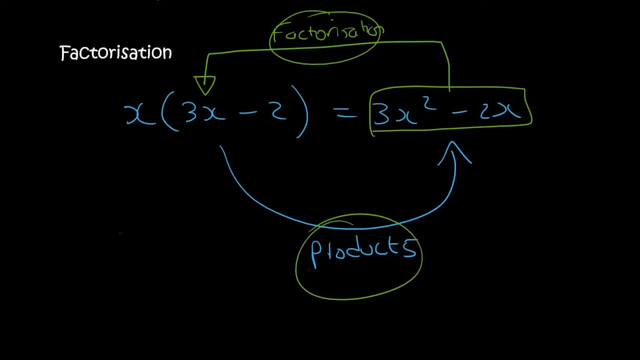 So factorization and doing the product are Opposites of one another. They are completely different, okay, So let me, let's practice and I'm going to show you how this works. It's going to be a little bit weird at first, but that's how maths is. 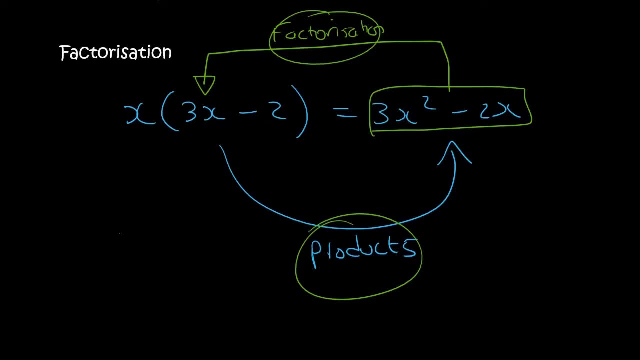 It's always a bit weird at first. In fact, that's how life is. Things can be strange, but then, as you practice it, you become better. And so you must practice, that's all. Once you practice, you become better. 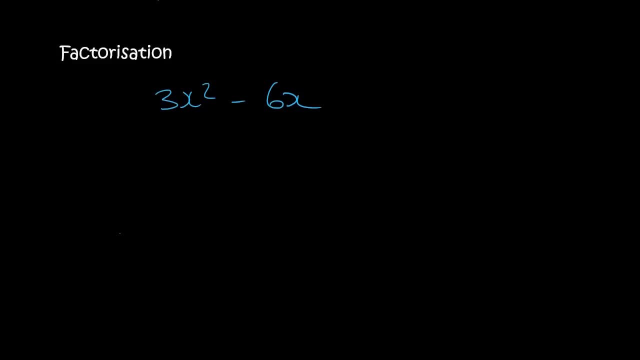 Easy as that. So here we have 3x squared minus 6x. So what we need to do is: Well, I'm going to, I'm going to show you a couple of examples and you will start to get an idea of how it works. 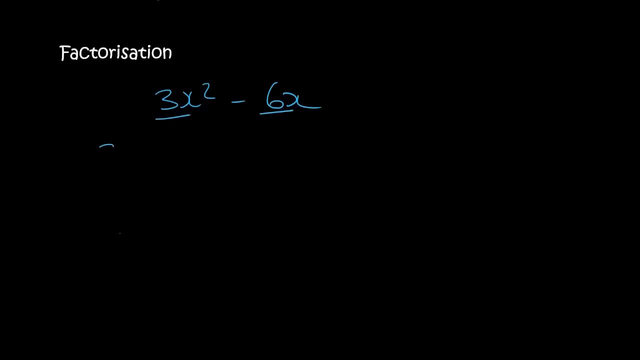 So I know that the number 3 can fit into both of these, So I'll take that out in the front. I also know that this one here has 2x's and this one has 1x, And so I can take out 1x. 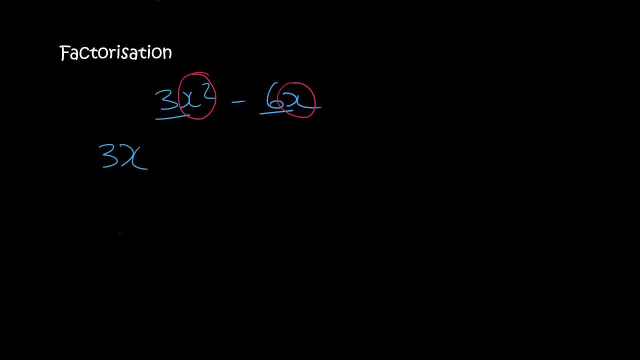 Because they have that in common. okay, They have 1x in common. Then we need to see what is left over. So in this first term there's still an x left, And then we're going to say minus 2.. 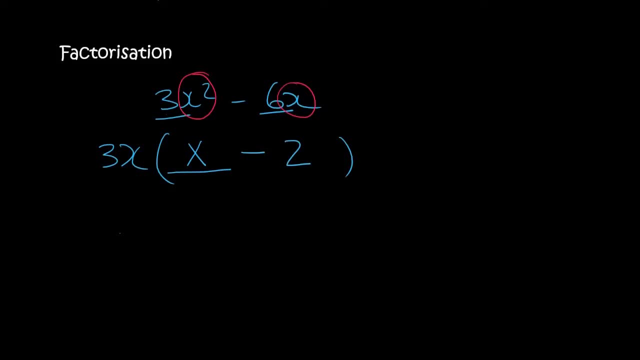 Now, if it feels a little weird right now, of course it will. It's a brand new topic Now. this is the answer. But let me prove it to you. If I gave you this question and I said, please find the product, you would multiply this in. 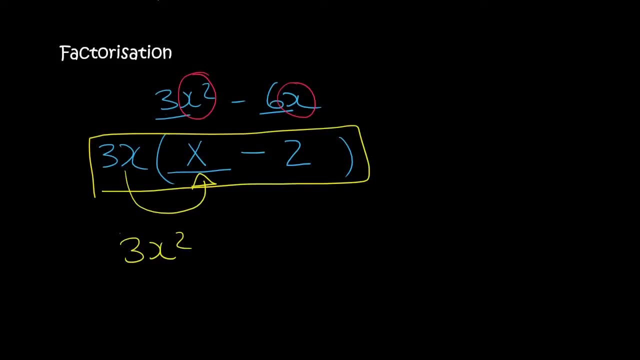 And that would give you 3x squared. You would then multiply this in and that would give you minus 6x, And so we are back at the original question. And so if you are asking If you are asked to factorize 3x squared minus 6x, this is the answer. 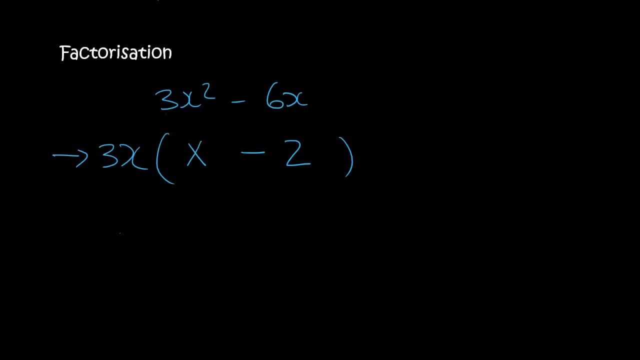 Let's practice a lot of examples and you'll start to become more familiar. So, with this one, the biggest number that they have in common is a 10. They have 2x's in common. Then what will be left? 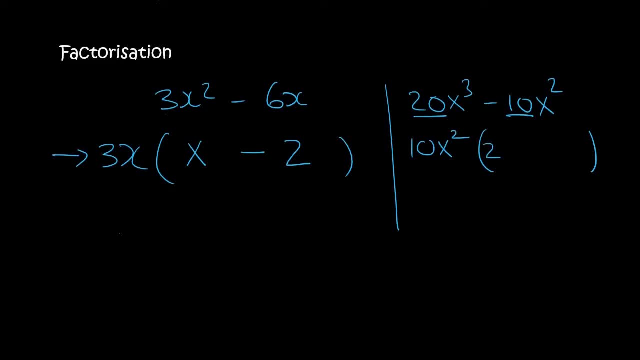 Okay, So for this one you would still be left with a 2, and there's still one more x left over. With this one, there's nothing left over, so you just say minus 1.. Let's see if this works out. 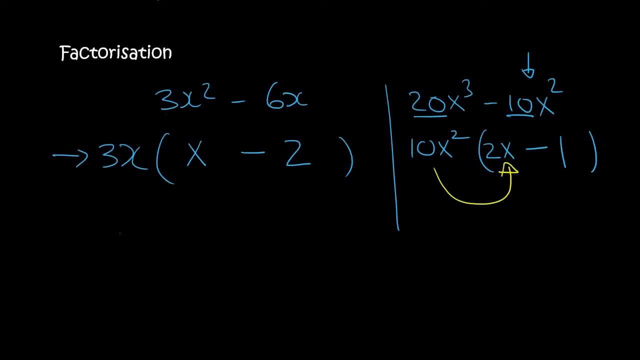 So if you had to multiply this back, that would give you 20x to the power of 3, minus 10x squared, which is what we originally had. So the answer is this over here. If you want, you can pause the video and try this yourself. 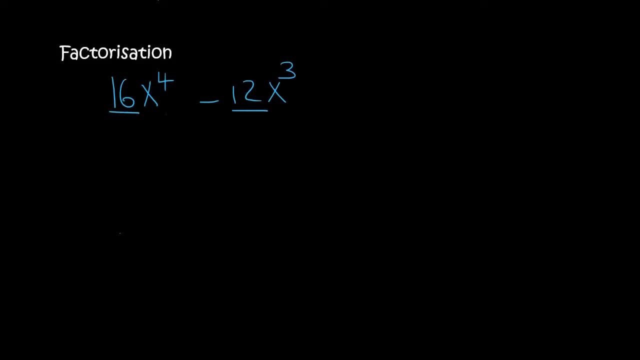 So the numbers 16 and 12, the largest number or the largest multiple that they have? Well, not multiple. The largest factor that they both have Is a 4.. Then there are 3x's in common, because this one has 3x's, this one has 4, and so they at least have 3x's in common. 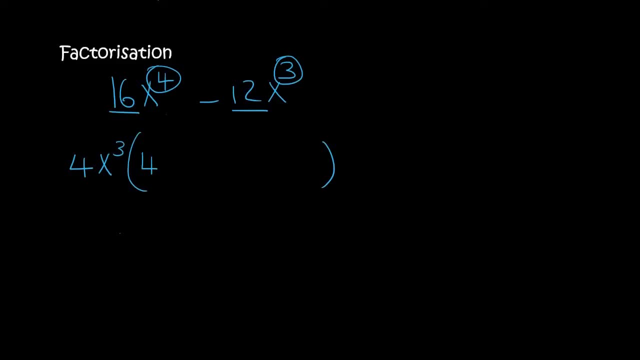 Now let's see what's left over. Well, there will be a 4 left over here and an x, and then this will just be minus 3.. Because if I had to multiply this back, you would get 16x4, and 12x3.. So the answer Is that over there. Okay, So with number 1.. The largest number, that Well, the largest factor of both of those is the number 20.. This one has 1x, this one has 3.. So how many do they have in common? 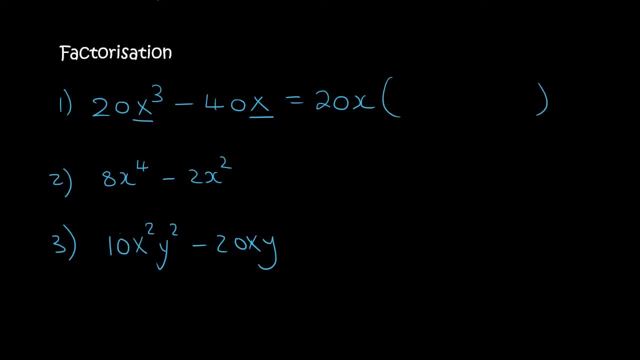 They share 1x in common, And so what will we be left with in the first term? Well, only an x squared, and then minus 2.. How do I know that that's correct? Because if I had to multiply this back, that would give you 20x3.. 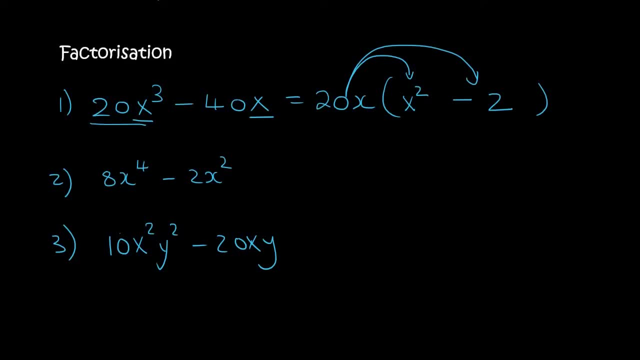 And if I had to multiply this you would get 40x. The next one, The largest number in common between an 8 and a 2, is a 2.. Then this one has 2x's. this one has 4.. 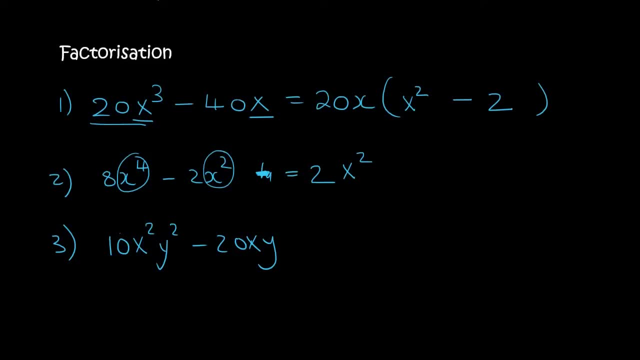 And so they can at least have 2 in common. We will then be left with 4x2-1.. Now, if there are any of you who are watching this for revision, then you will already know a factorizing method called difference of squares. 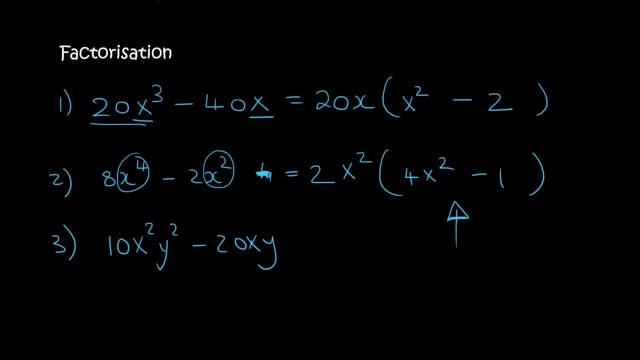 And so technically, this one could go further. But I'm just going to pretend that you are getting started with factorizing and so I'm not going to go further with that one for now. I didn't know that that one was actually going to turn into a difference of square. 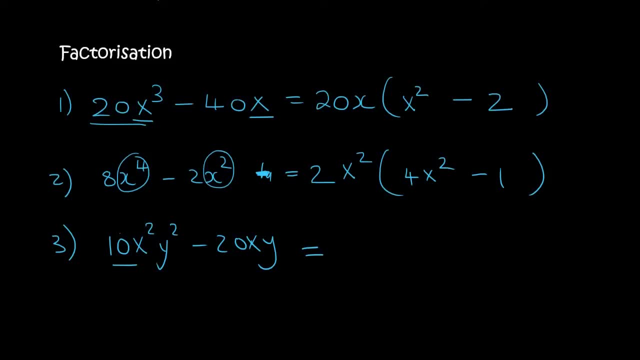 Now in the third one, the largest number that can go into both is 10.. Let's look at the x's. For the x's, there are 2 over there and 1 over there, And so how many do they have in common? 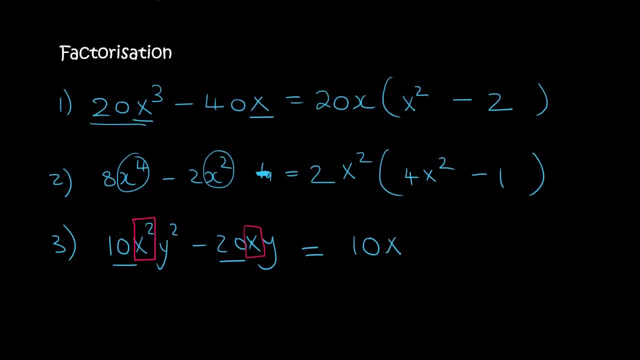 They've got 1 in common For the y's. there are 2 over there and there's 1 over there, So there's 1y in common, And so what you would be left with is, in the first term, you would still have an x and a y. 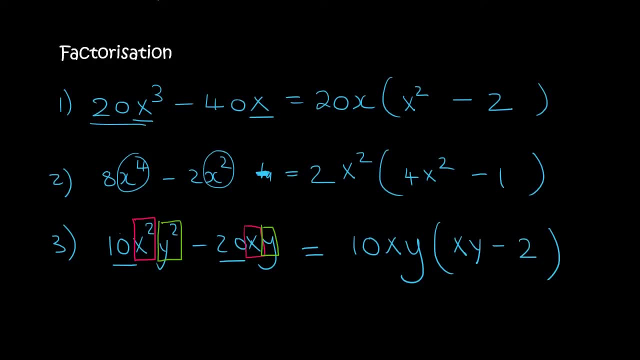 In the second term you would just say minus 2.. Let me show you that in a different way Now. this technique I'm going to show you now. I wouldn't advise you use it all the time because it would take quite long. 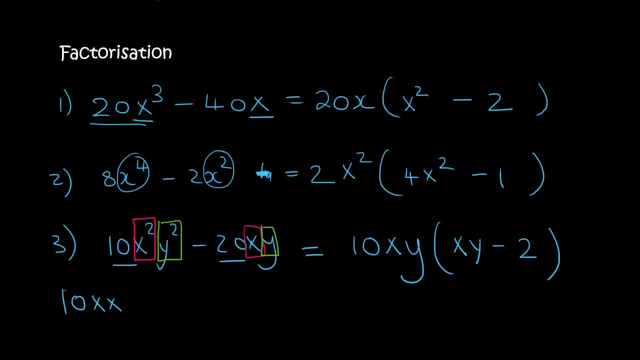 But 10x2 is the same as 10xx and y2.. y2 is yy, 20 is the same as 2x10, and then there's xy. So what things are in common? Well, there's a 10.. 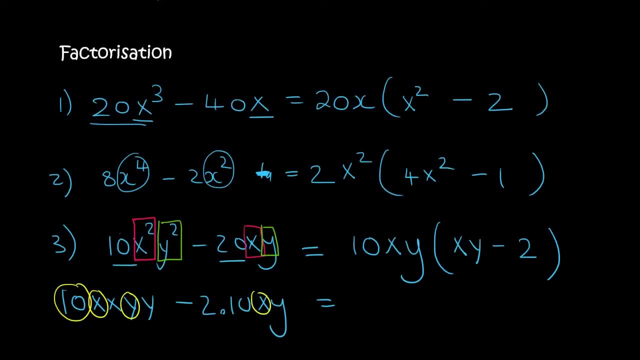 They both have an x And they both have a y. So that is why we take out 10xy. So let's do that quickly: 10xy. Now, what is left? Well, in the first term, we still have an x and a y. 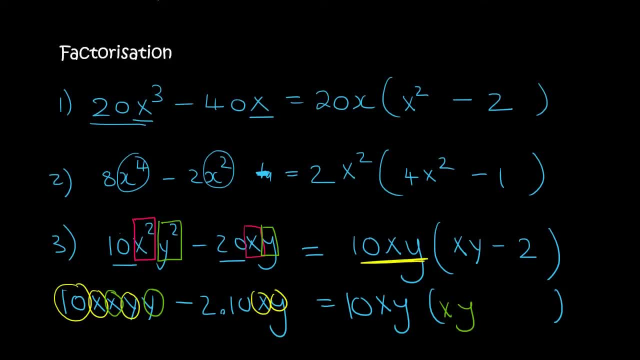 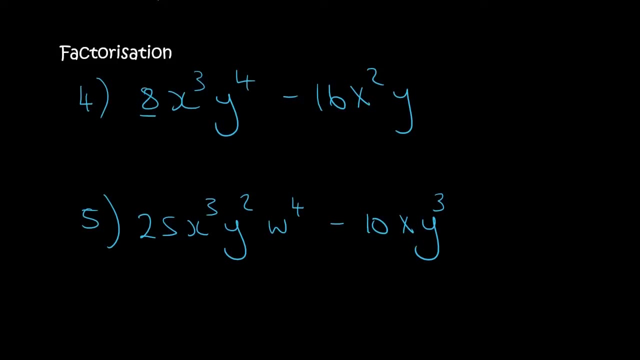 So we say xy In the second term. oh, we also took that 10,, Kevin. So we still have a minus 2 left over over here, And that is why we say minus 2.. So if you want to use that long method for now, just until you become more familiar with it, that's absolutely fine. 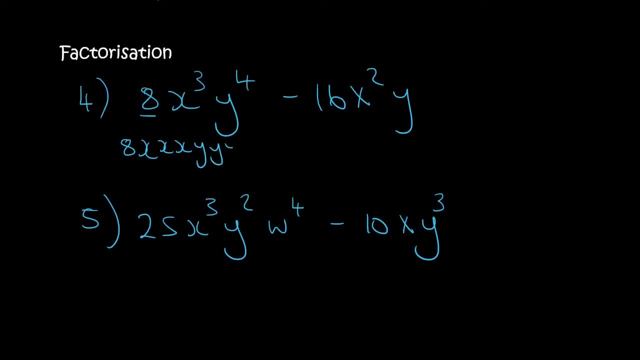 So this will be 8xxxyyy minus 2 times 8.. Because 16, you've got to sort of be able to see a common thing between them: There's an 8.. So then we can say that that is 2 times 8.. 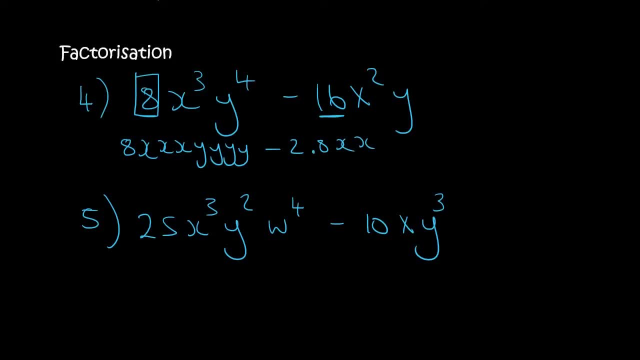 I'd rather write it like that. And then there's 2 x's and then a y, So the number 8 is common. So I'll circle that for both of them. They have this. one has an x, so it can go in common with that one. 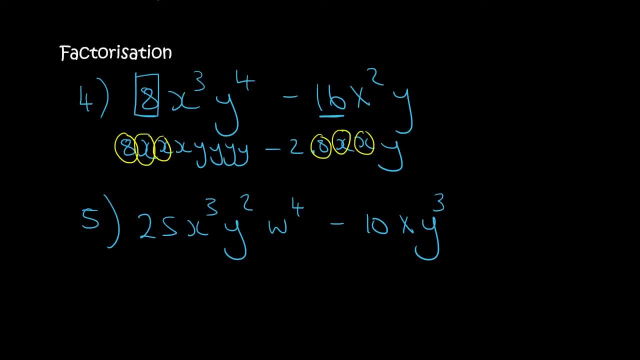 This one has an x, so it can go in common with that one. This y goes with that y. Okay, so that is what we can take out. We're taking out an 8. 2 x's- see there- And then a y. 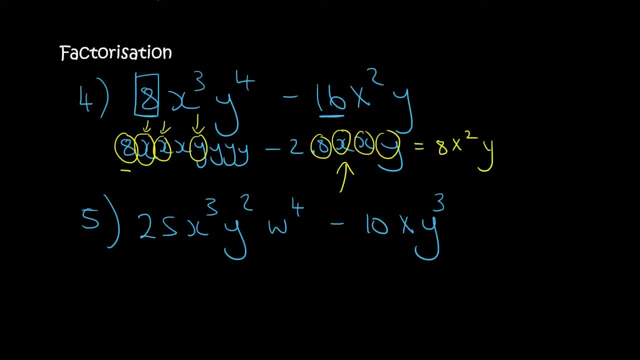 And that's the same for this one. There's an 8. There's an x squared and a y. Now we open up our brackets And what are we left with? Well, we are left with an x and then 3 y's. 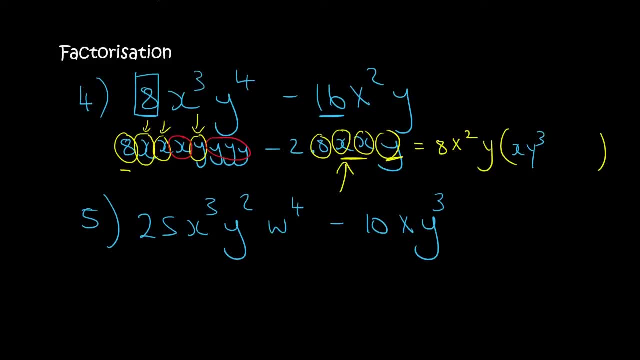 So that will be xy3.. What are we left with? in the first term, Minus 2.. Like that For the next one. well, straight away, you should know that 25 and 10 have the number 5 in common. So you're going to break this up into 5 times 5.. 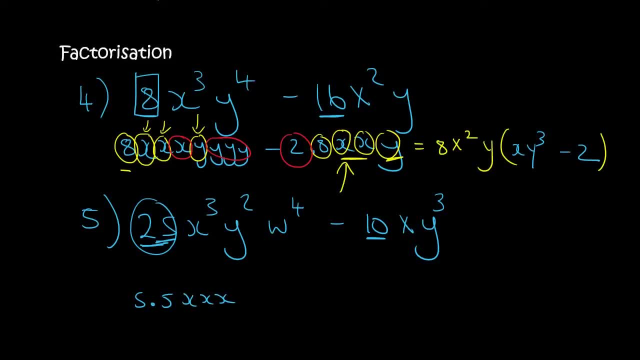 Then 3 x's xxx. You see why this method could get really long, Because if I start saying x10, then you're going to have 10 x's next to each other, Then yy, and then 4 w's, Then 10 is going to be 5 times 2.. 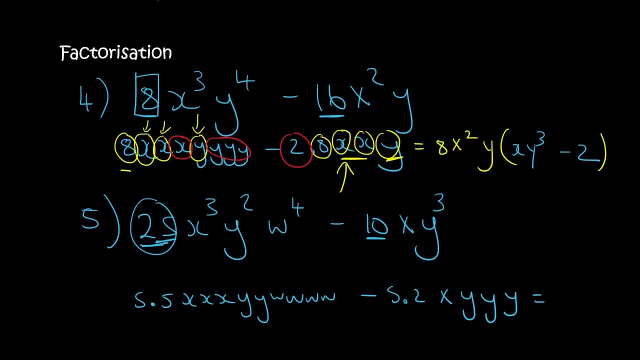 There's 1 x and 3 y's, So let's see what's common. So this 5 is in common with that 5.. This x with that x, And then this y with that y And this y with that y. 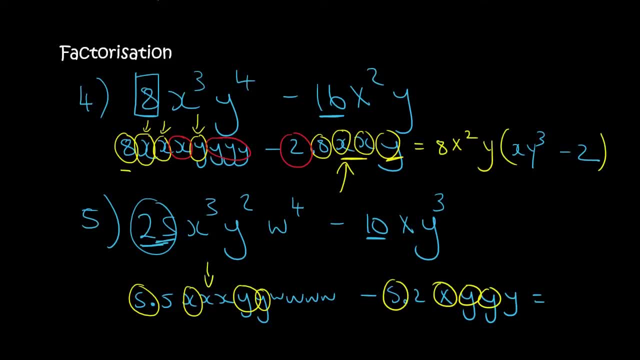 Then there's nothing else in common. For example, I can't choose this x because then I don't have a matching partner on the other side, And so the common- sorry that y fell away. So the common thing is a 5, an x and then 2 of these y's. 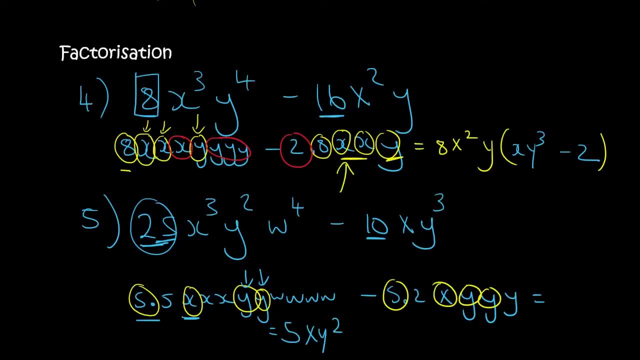 That will be y2, and I'm running out of space. Okay, so I took out a 5xy2.. Now let's see what's left. In the first term, we still have a 5 and then 2 x's. 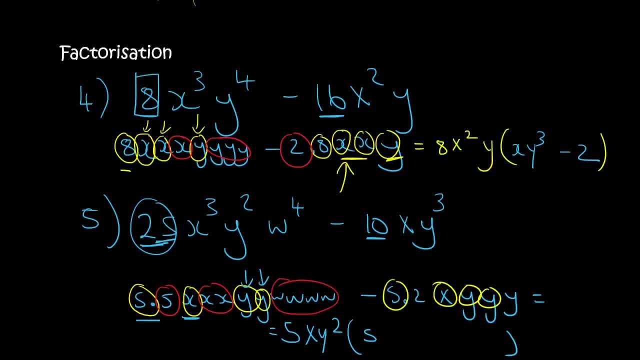 And 4 w's, So that will be 5x2 and then 4 w's. In the second term we still have a 2 and then a y, So that will be minus 2y, And there's your answer. 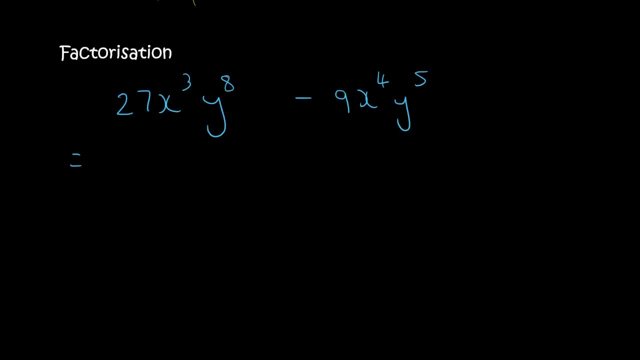 And so let's try to do it without writing out all those numbers like that. So what number can we take out of a 27 and a 9?? Well, you can take out 9. You want to take out as much as you can. 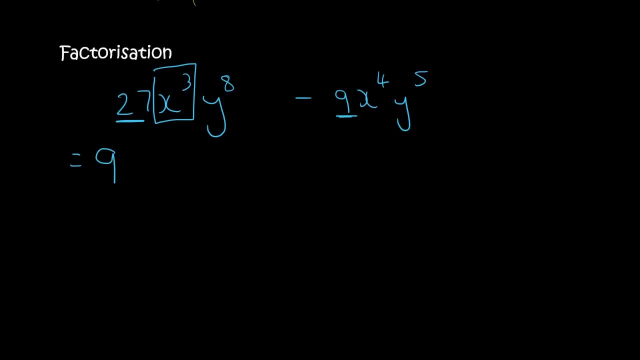 Now imagine this xxx, so 3 x's. This one has 4 x's, So it would look like xxx, This one would be xxxx, And so the common ones would be: that one goes with that one, That one goes with that one.